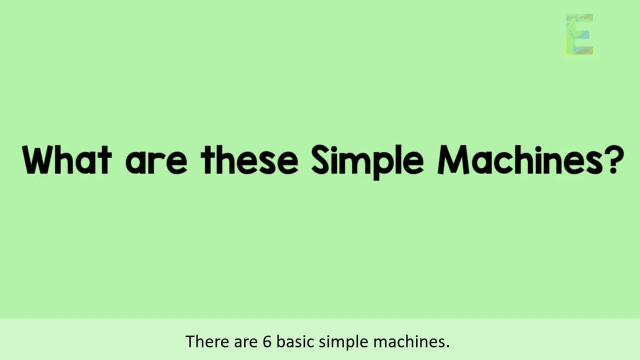 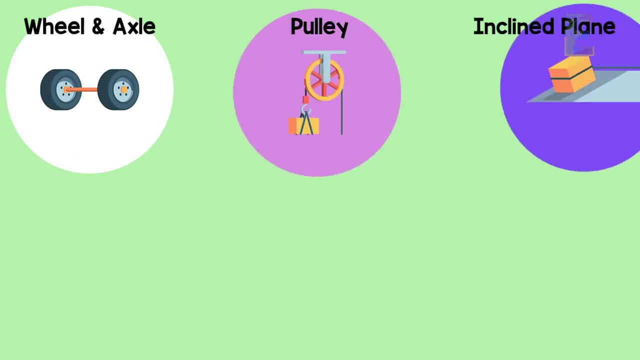 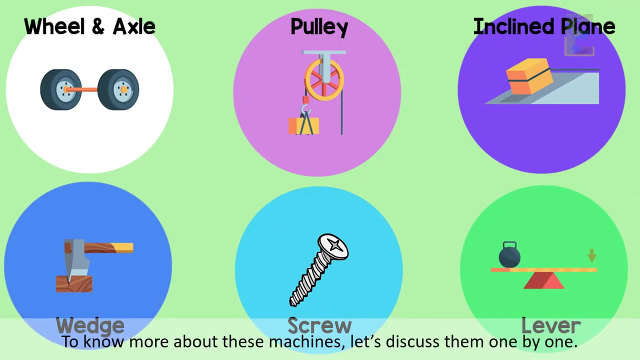 these simple machines. There are six basic simple machines. These are wheel and axle, pulley, inclined plane, wedge, screw and lever. To know more about these machines, let's discuss them one by one. Let's start with wheel and axle. 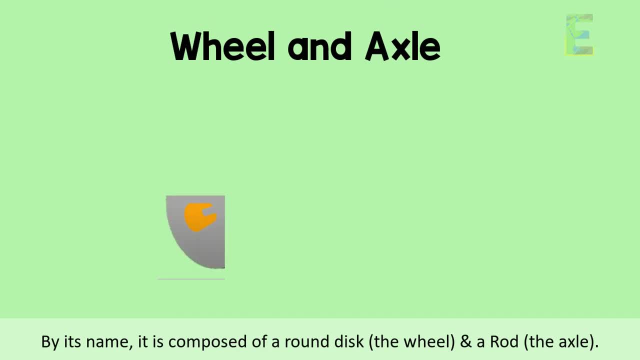 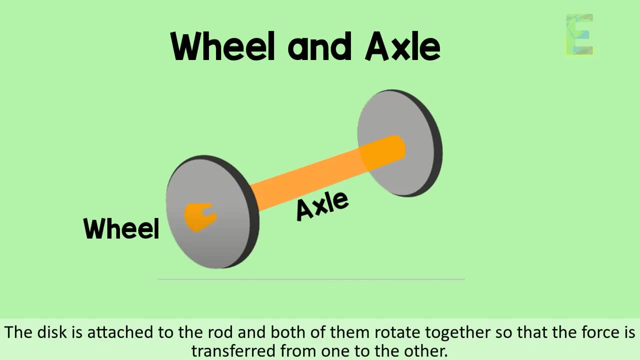 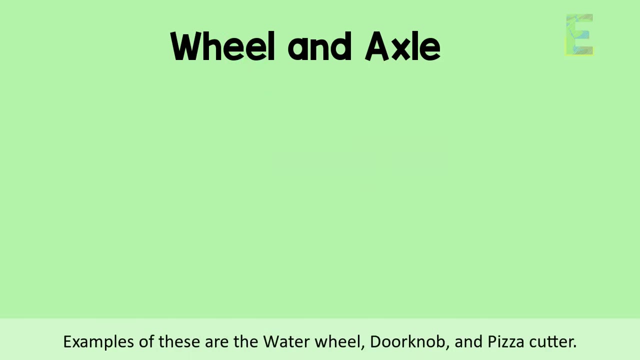 By its name. it is composed of a round disc, or the wheel, and a rod or the axle. The disc is attached to the rod and both of them rotate together so that the force is transferred from one to the other. Examples of this are the water wheel, door knob and pizza cutter. 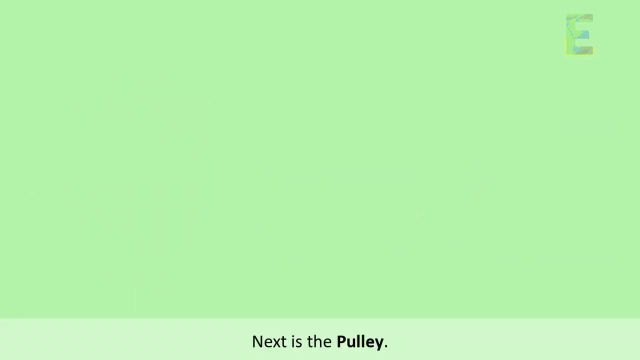 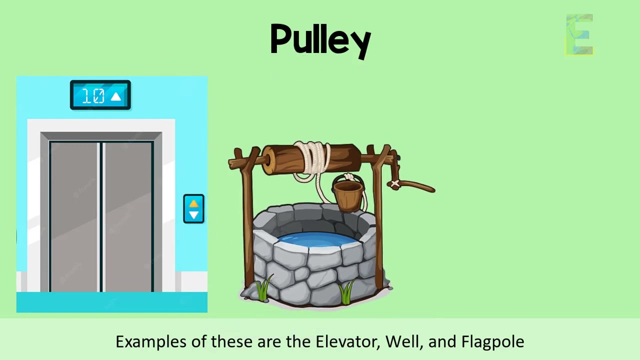 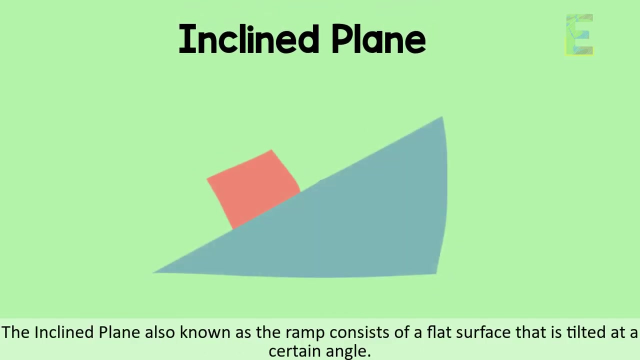 Next is the pulley. Pulley is composed of a wheel and a cord. the wheel rotates and carries the cord. examples of this are the elevator, well and flagpole. the third is the inclined plane. the inclined plane, also known as the ramp, consists of a flat surface that is titled at a certain 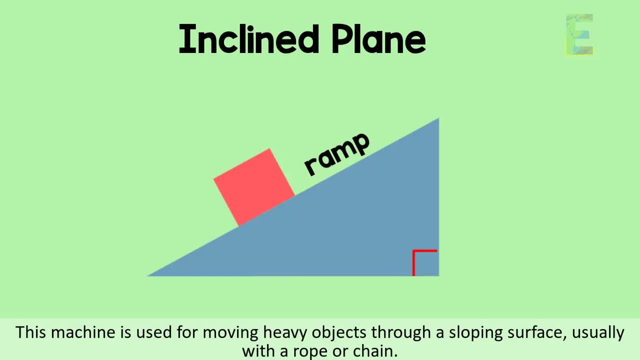 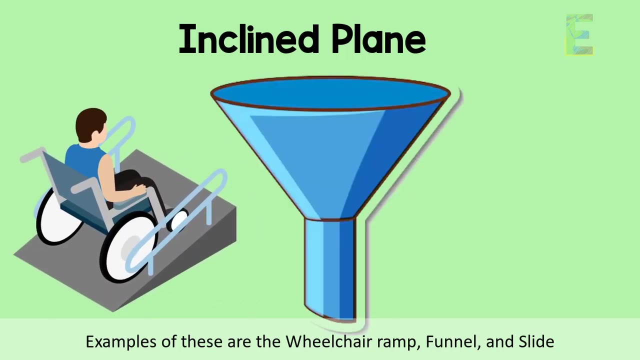 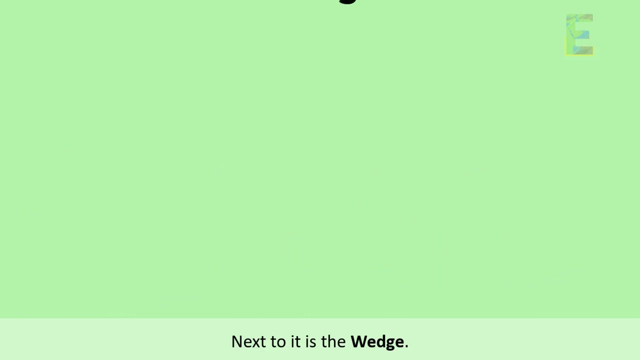 angle. this machine is used for moving heavy objects through a sloping surface, usually with a rope or chain. examples of this are the wheelchair ramp, funnel and slide. next to it is the wedge. a wedge is basically a triangular shaped object. on one end it is thick and thin or sharp. on the other it is used to 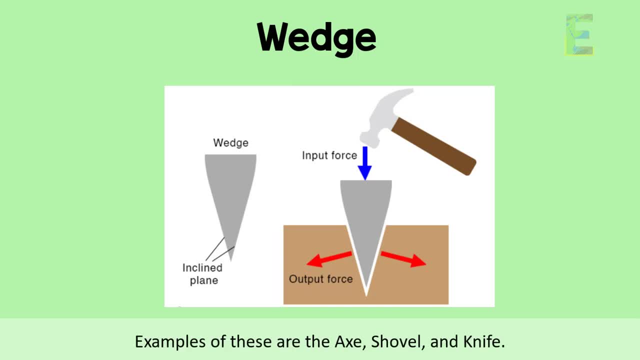 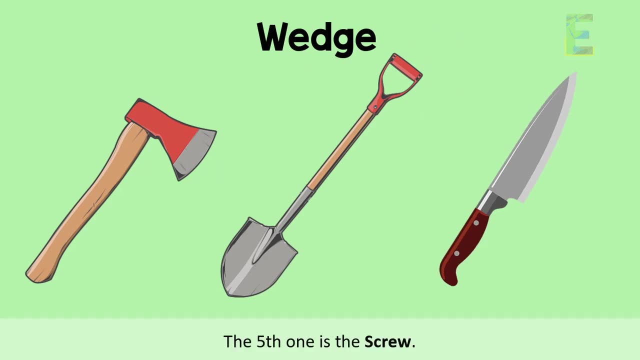 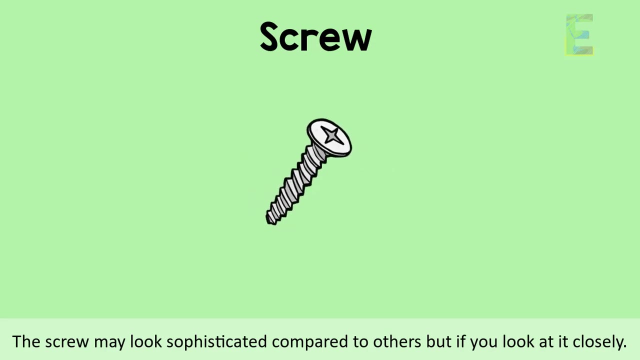 split things into pieces. examples of this are the axe, shovel and knife. the fifth one is the screw. the screw may look sophisticated compared to others, but if you look at it closely it is just a wedge wrapped around a cylinder rod. its mechanism is it? it converts rotational motion into a linear motion. examples of this are the: